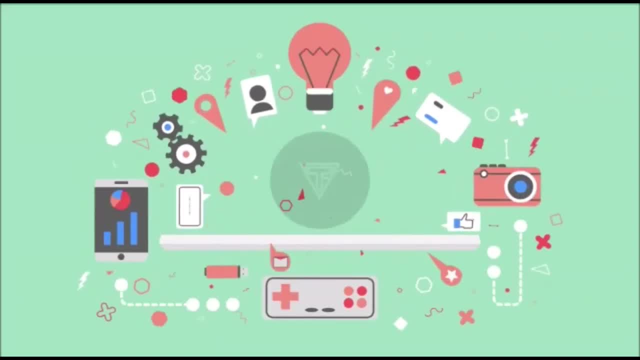 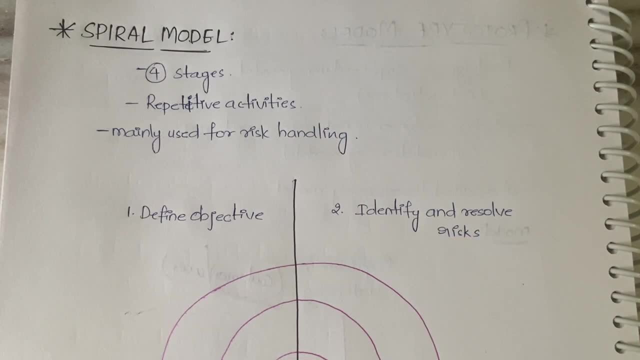 Hello everyone, welcome back to my YouTube channel, Trouble Free. In this video, I am going to explain you about spiral model in the subject of software engineering. Till now, we have discussed about different process models, and the spiral is the second one in the iterative model. 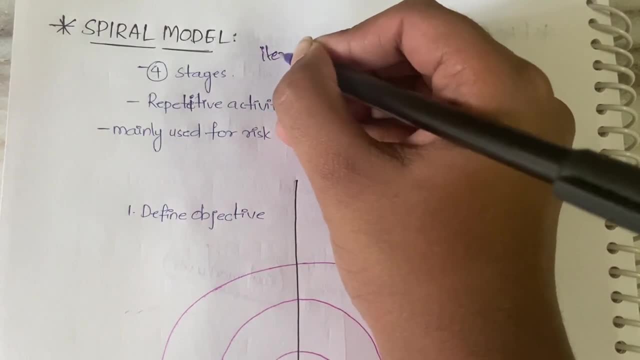 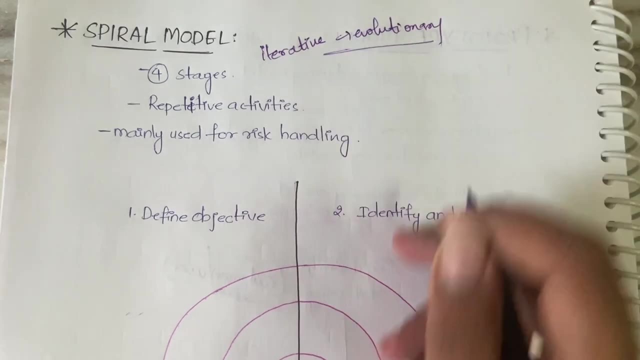 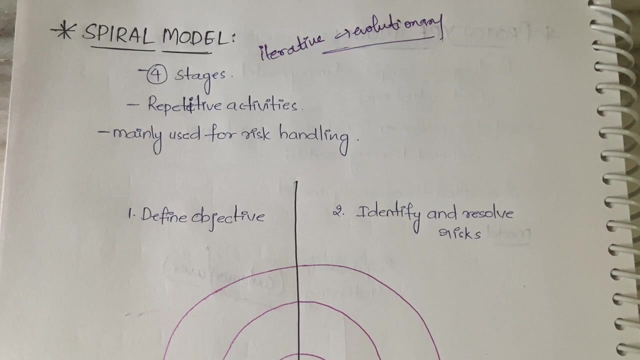 Okay, so it comes under iterative process model, and iterative process model will come under evolutionary process model. You already know that, right, Okay? So before that, yeah, one more thing. I've started a new channel with study abroad content. If you're having interest, I'll leave the link of that channel in the description. You can have a look. 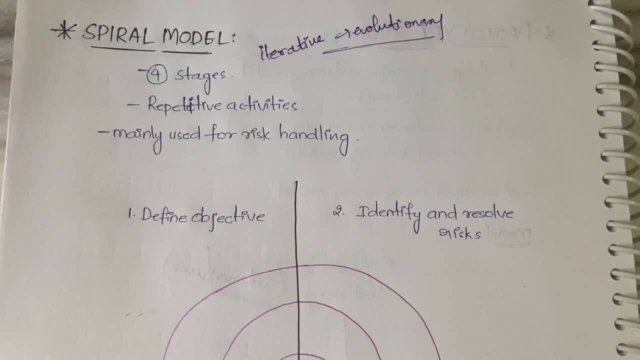 So now let us see this spiral model. So it actually has four stages. It is an endless loop, So it never ends. I mean, it ends when you want it to end, Okay, that's okay. Don't get confused, I'll explain you. 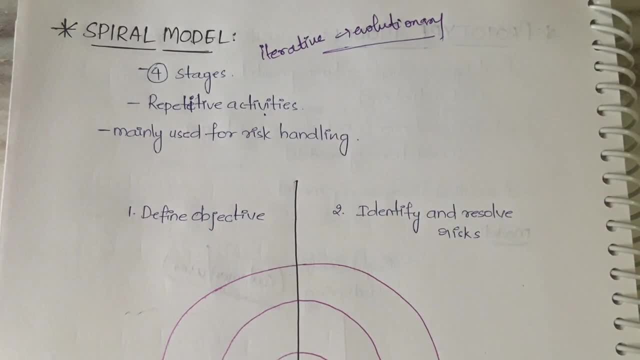 So all the repetitive activities will be done, That is, each and every activity will be repeated multiple times until the customer is satisfied. And it is mainly used in case of risk handling, or you can simply say, in case where handling risks is very important or in the cases where more risks are probable to happen. 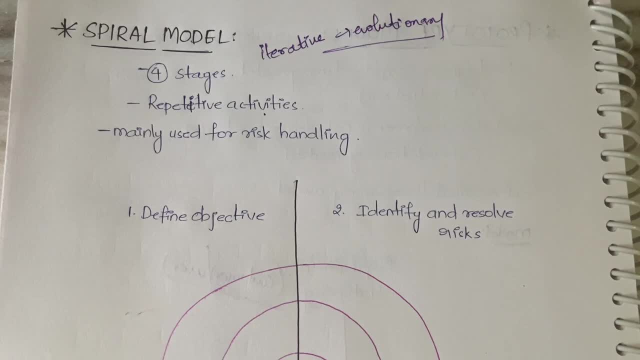 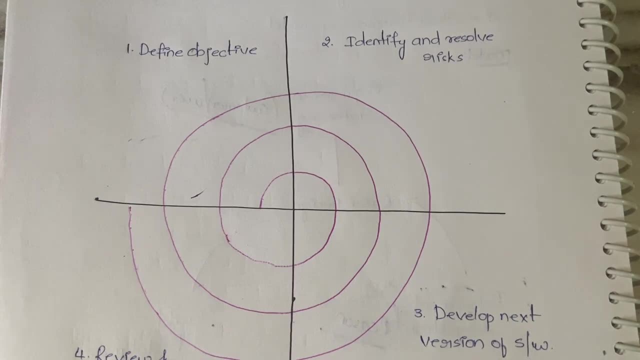 So in those cases you can use the spiral model, Okay, Okay, So now let us see the diagram with which you can understand it more clearly. Okay, I think I cannot zoom in more. If I zoom in more, it is becoming blurred actually. 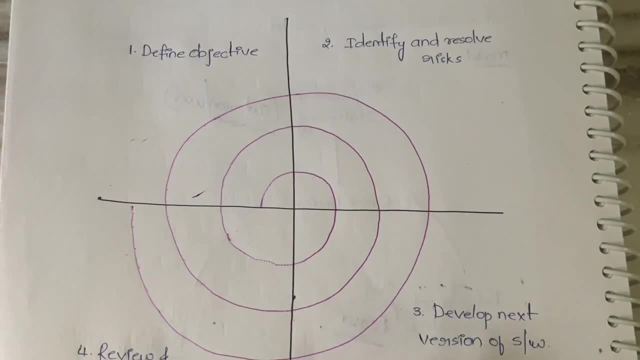 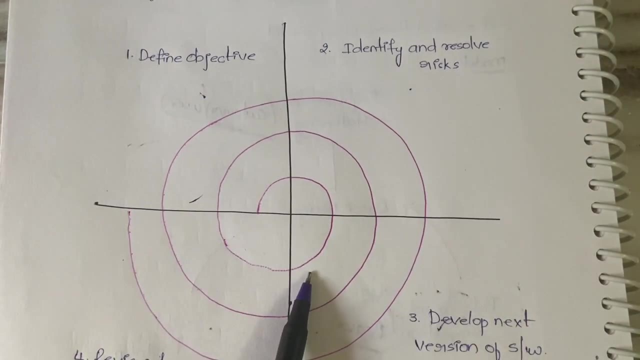 0.96.. Okay, fine, Let us keep it on one only. So this is the diagram. We have four stages, four quarters: 1, 2, 3, 4.. Okay, So don't get confused. in coordinate geometry We'll have 1,, 2, 3, 4, but here 1,, 2, 3, 4, like this We have Okay. 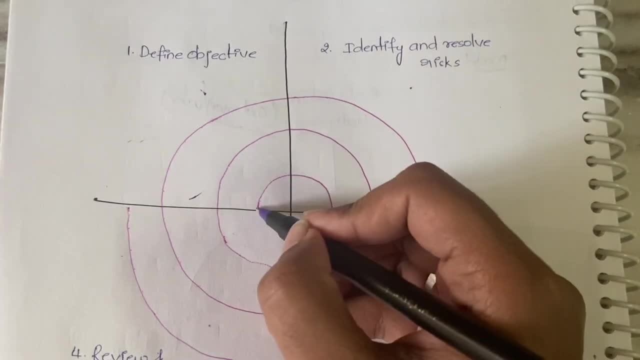 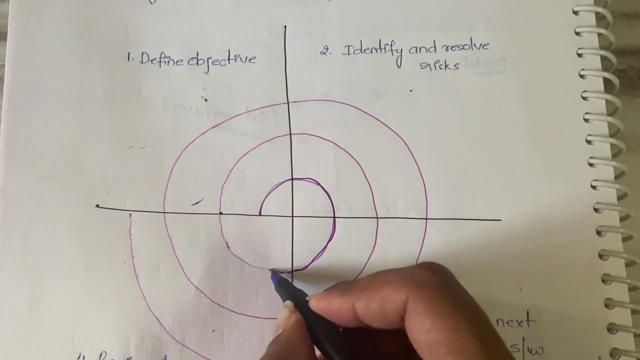 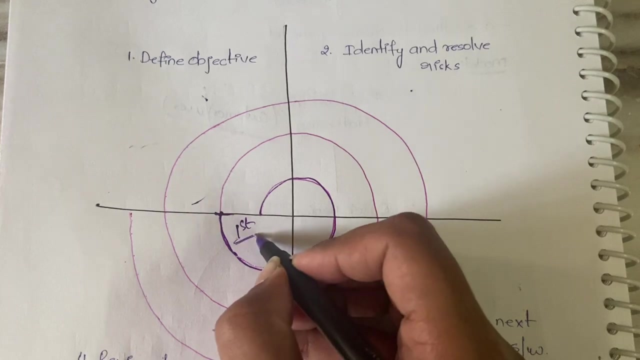 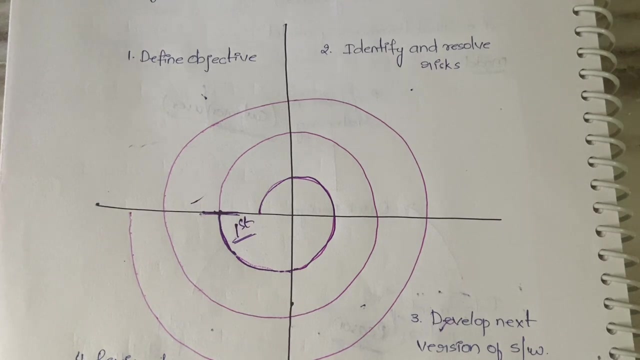 And in this direction it comes. So see, it is starting here and one complete cycle It'll make. sorry, Okay, By the time it comes here, one complete cycle is completed. That is first iteration is done, Okay Now, if so, here it reaches. first iteration is done with. then the customer will come, He will evaluate, He will check if the customer is not satisfied. 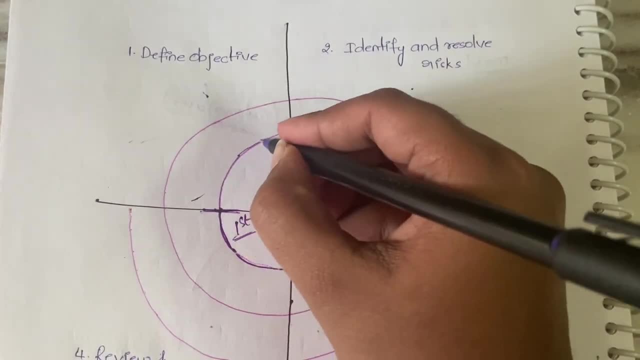 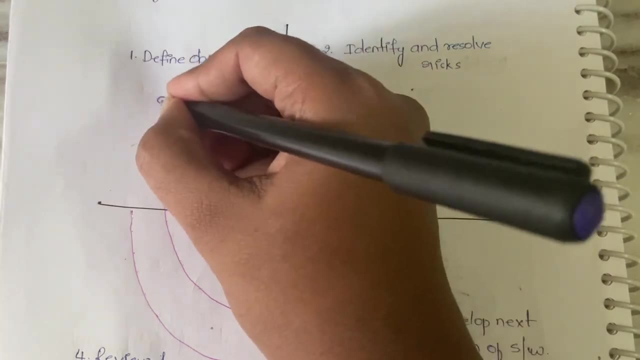 It will go for the second iteration. Okay, that is in this way. okay, so here it starts from here. always it will start in q1 and end in q4. okay, see, here it has started here and ended here. right now again it is starting here, the second. 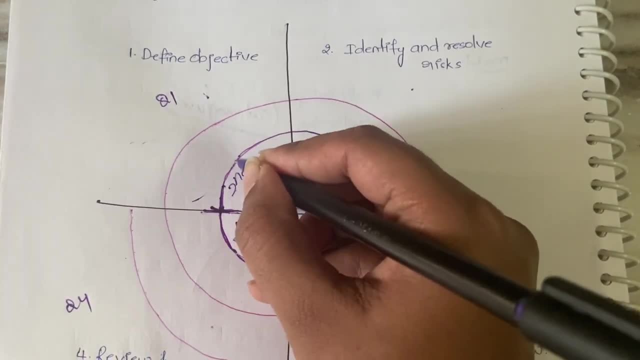 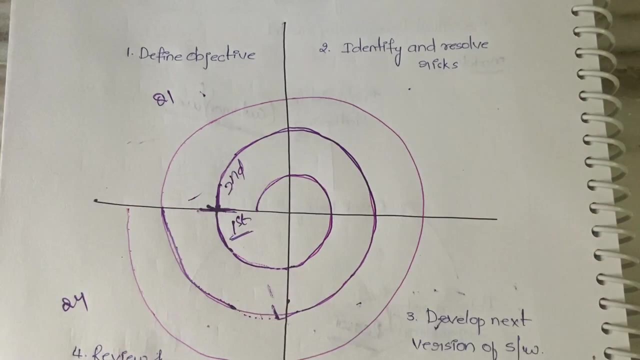 iteration is starting here in q1, and it will travel all the way and it comes here and stops here. okay, q4, like that. again. here also, customer evaluation will be done if the customer is not satisfied. one more iteration like that. the spiral with the loop continues until and until the until. 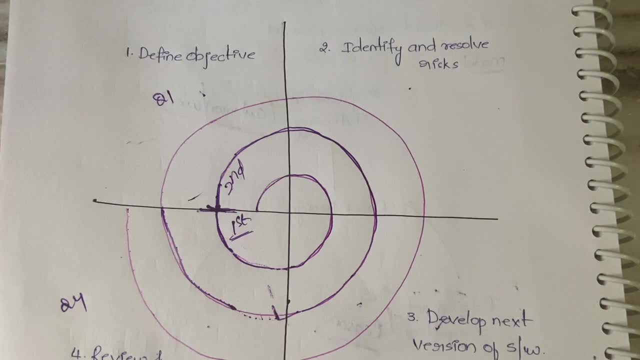 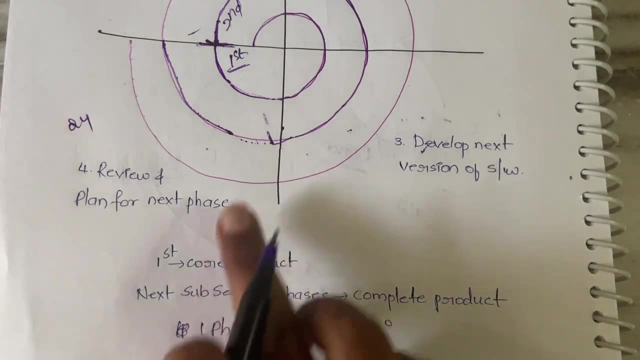 and unless the customer is satisfied. okay, so we have four steps here. i will tell what are those four steps. before that, let us see some more features of this spiral model. so the first iteration. so the first iteration is the core product and in the next, subsequent iterations. 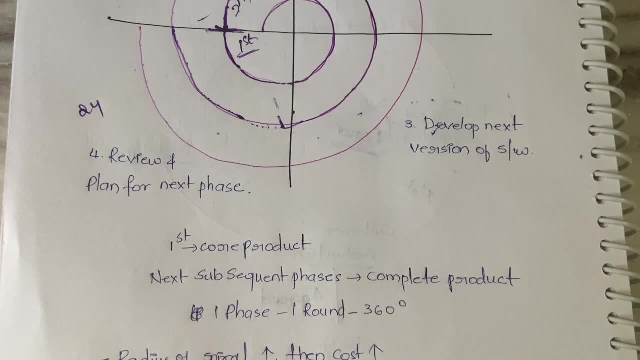 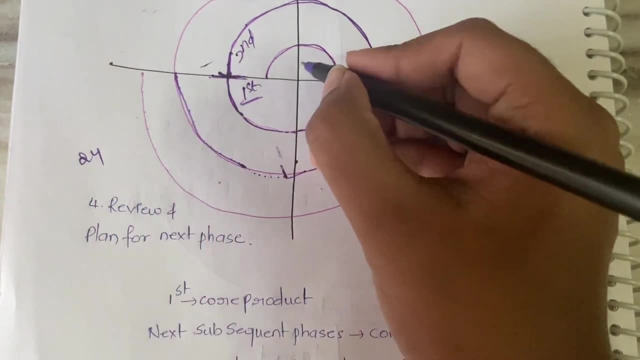 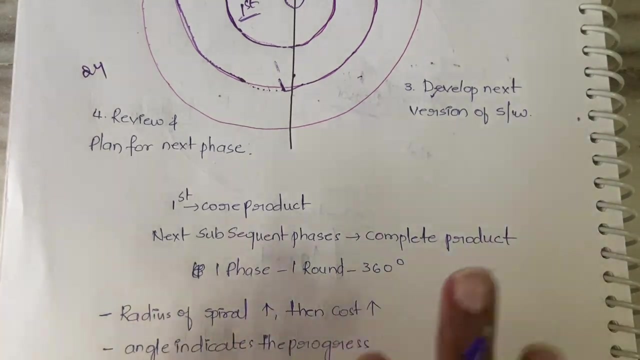 you will be getting the, a final complete software. okay, subsequent phases, faces is nothing, but one phase is 1 round. okay, one round is one phase. one round in the sense: complete, this one, this complete 360 degrees, is considered as 1 round. okay, as radius of the spiral increases, cost also will. 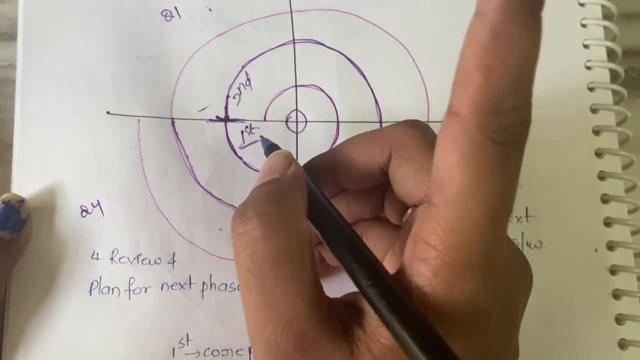 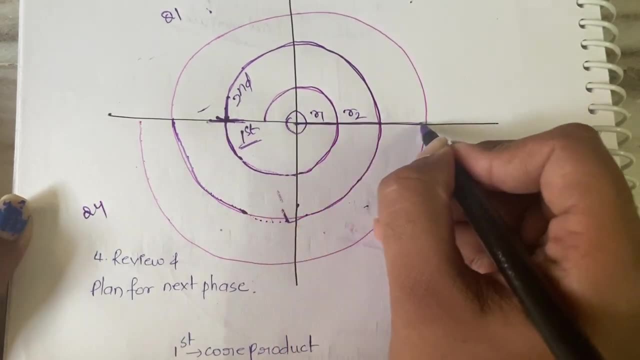 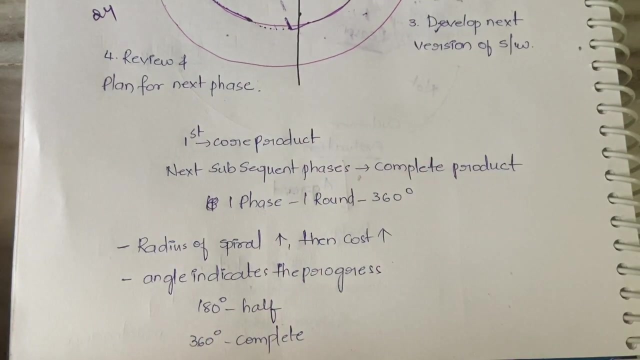 increase radius of the spiral in the sense. so what is the radius of the first iteration, this one- r1. what is the radius of the second iteration, this- r2- what is the radius of the third iteration- r3? so, as the radius keeps on increasing, cost also will increase, okay, and the time also will increase, the complexity also will increase. 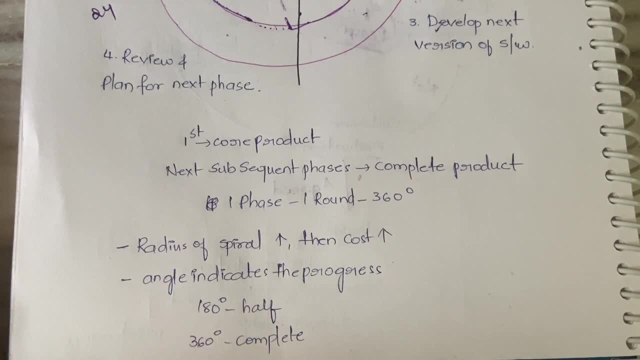 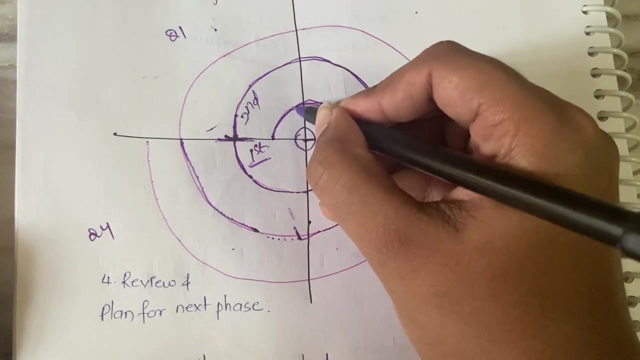 everything will increase as the radius of the spiral keeps on increasing, okay, and the angle will indicate the progress. so what do you mean by the angle? suppose it has traveled in this way, okay, so how many? how much angle? it has covered 180 degrees, right, so half of the task is done. 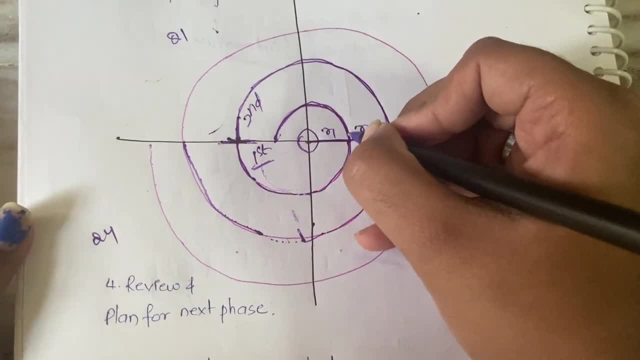 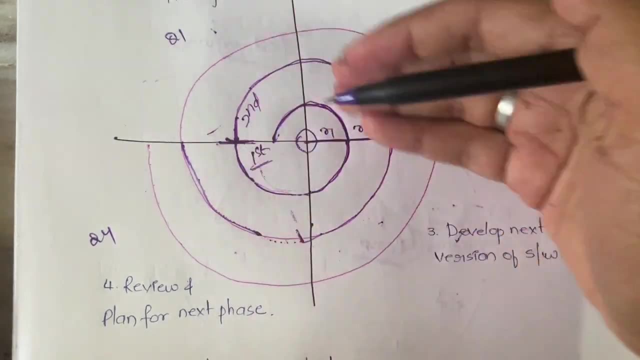 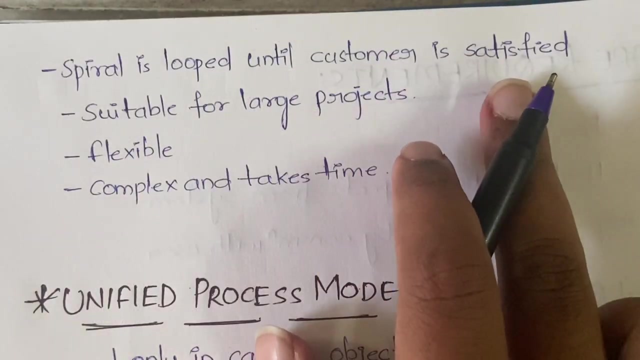 more half is yet to complete support it, it has traveled this way. then 270 degrees, that is three-fourth of the task is completed, one-fourth is more lift. like that, the angle will represent the progress of the task. got it so, and now i really is looped until the customer is satisfied. 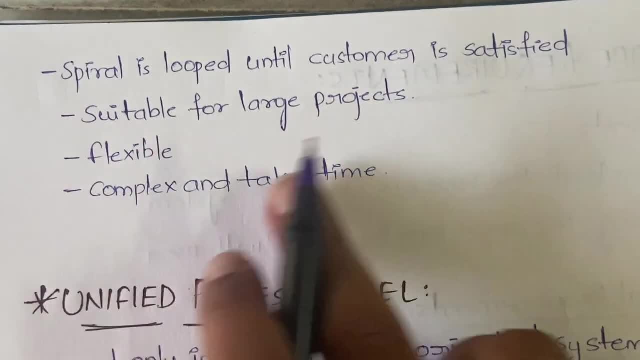 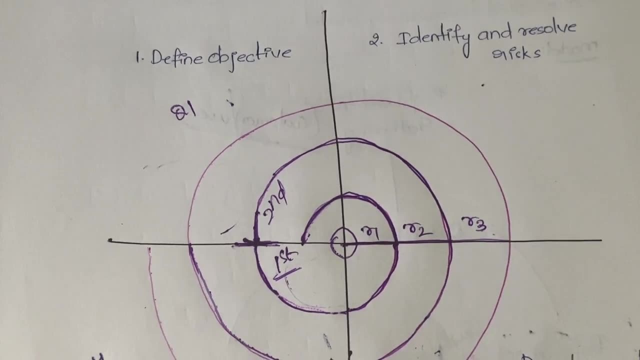 it is suitable for large products projects and it is also flexible and it is compli complex, obviously, and it will take some time. okay, now let us see the diagram. that is, we have four stages, right? let us try to understand what are those four stages? very simple, they are, don't worry. first is defining the objective, so 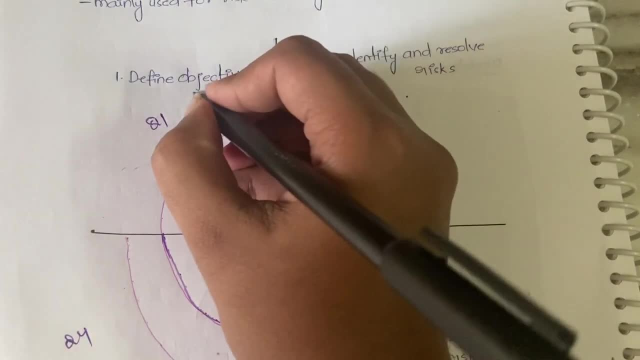 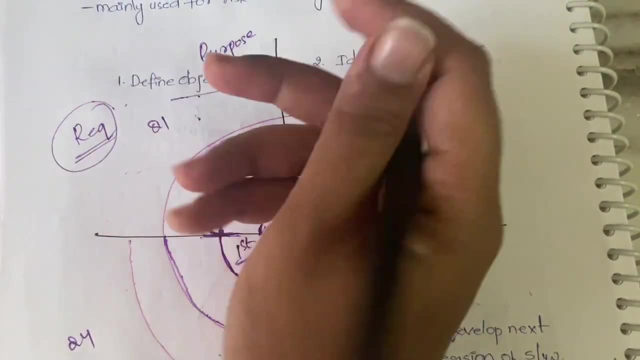 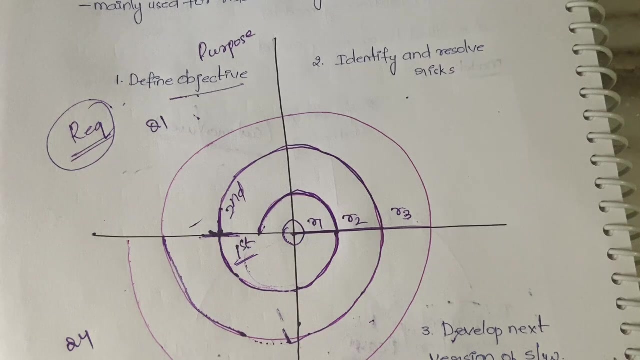 defining the objective. in the sense, it is nothing but the main purpose of the project. the main purpose why? how you will be able to define it? through collecting the requirements, through gathering the requirements. you have to define the purpose of the project, the objective, okay, and from there you move to the second. so, initially, what you are doing in the first phase. 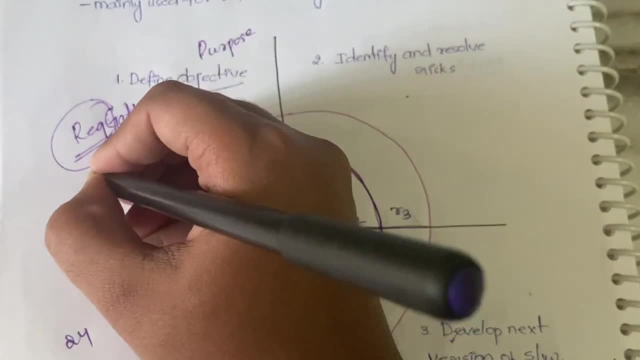 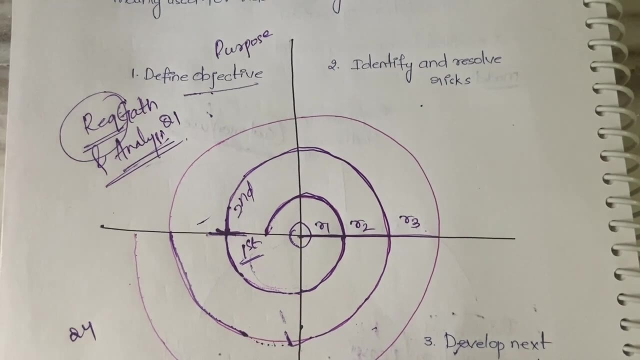 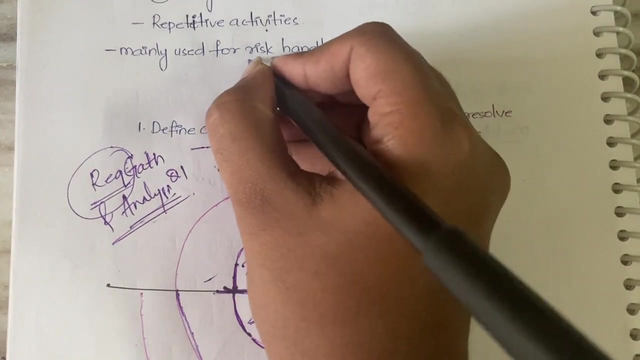 simply: requirement gathering and analysis. okay, next second: identify and reduce the resolve the risks. so in the second stage, what you will do is you will identify all the risks because, as i already said, this is mainly useful in case of risks. so the second step is you will identify all the risks and you will try to resolve those risks. 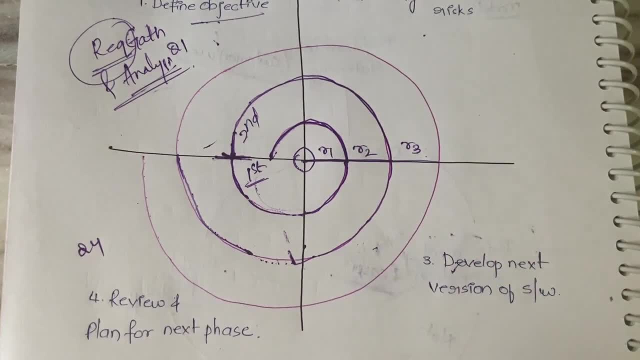 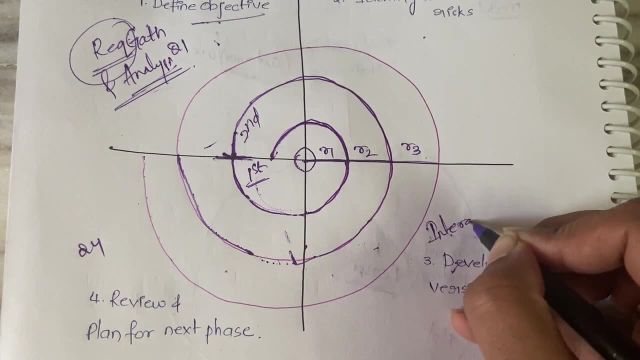 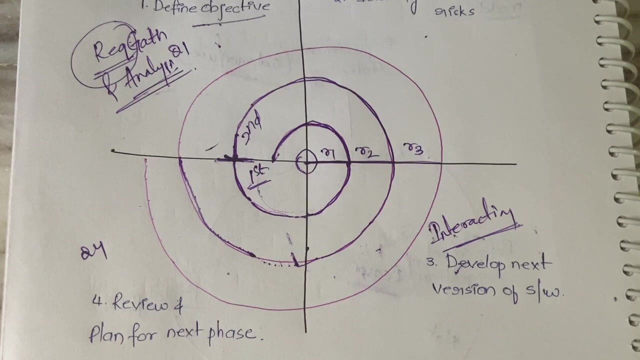 okay, then you will come to the third stage, which is nothing but the developing the next version of the software. developing next version of software is nothing, but you will be interacting with the customers. okay, interacting with the customers, and you will be taking the feedback from them. if there are any changes to be implemented, you will be implementing those changes.